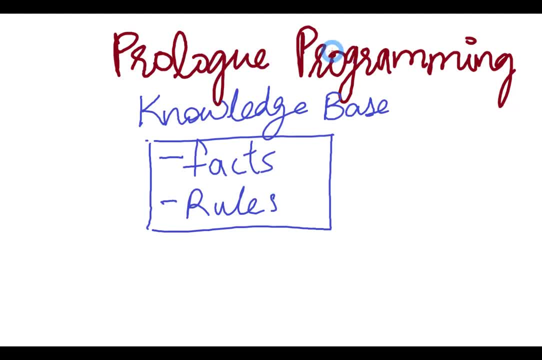 Let's learn about some basics of prologue programming. So in prologue programming we have a knowledge base, and knowledge base is just a set of information that you are given with, that you are provided with. So a good example can be human brain. So human brain is a knowledge base that has all the knowledge or information that it has acquired so far. So you have all the knowledge information that you have acquired so far and you use that knowledge, that information, to make different, different decisions in your life. So 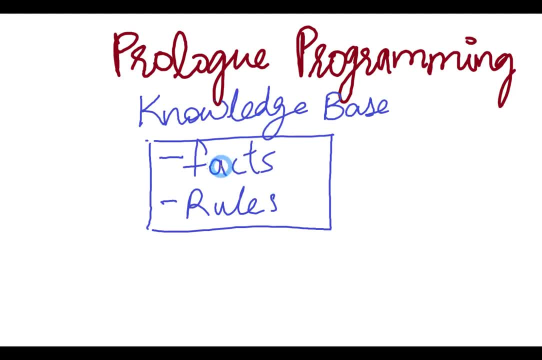 a knowledge base in prologue programming further comprises of two things: fact and rules. So facts are different statements that are true and rules are different statements that are based on facts. So, for example, a fact can be, So a fact can be: apple is a fruit and another fact can be: orange is a fruit. 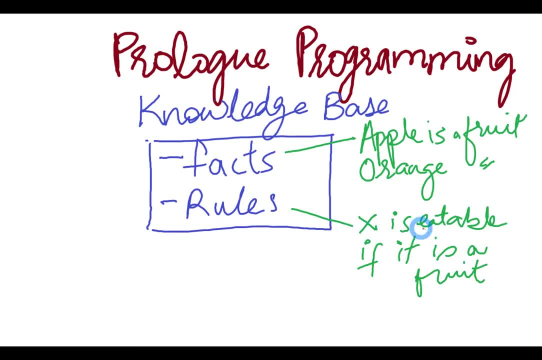 The example of rules can be: anything X is eatable if it is a fruit. So these two are facts and this is a rule: that anything is eatable if it is a fruit. Now, based on these facts and rules, we make different queries from this knowledge base. 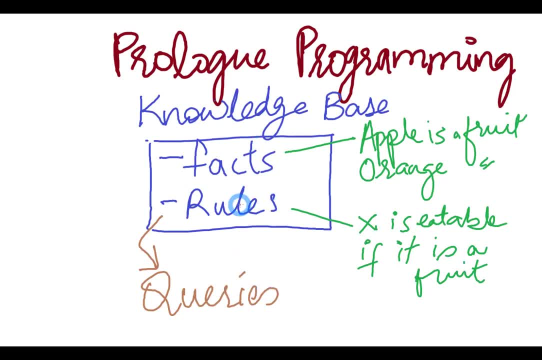 So, for example, we can ask this knowledge base, we can make a query that orange is eatable or not. And we have a fact for orange and we have a rule And so since the rule says that anything X is eatable if it is a fruit, so we will see whether orange is a fruit or not. we will see what is the. 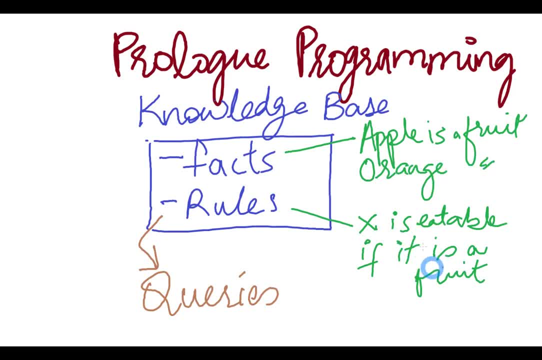 output true or false. so if orange is a fruit, that means it is eatable, right? so this is just a gist of it. let's see it in more detail and let's see the syntax and how will we implement it. how will we write a prologue program? 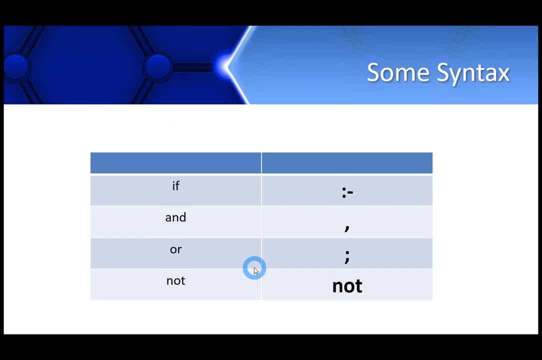 now let's come towards the syntax of prologue program. okay, so this is the syntax of some very basic words in prologue and you should always remember it if you're writing programs in prologue. so for, if we use the symbol colon and hyphen for and we use comma for or we use the semicolon, 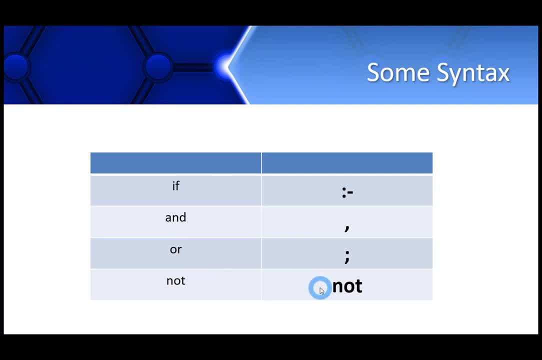 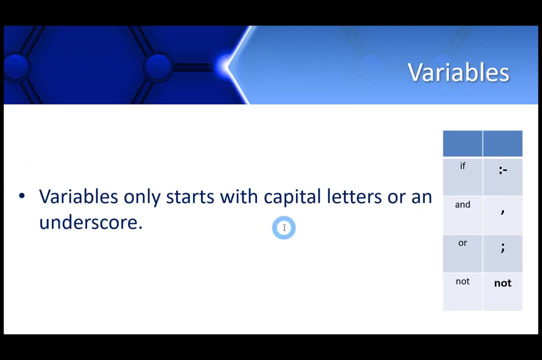 and for not. we use the keyword not right now. let's begin by learning about variables. so, in prologue, variables always start with capital letters or an underscore. so a variable can be single letter, but it will always start with a capital letter or an underscore. so in case it is, 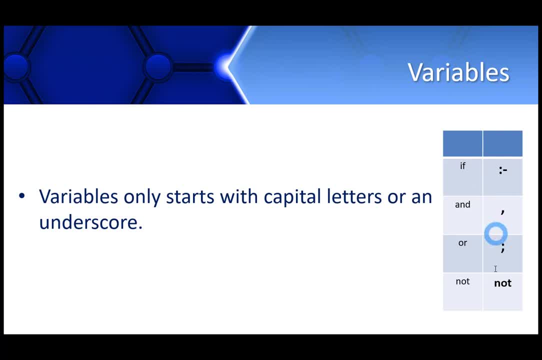 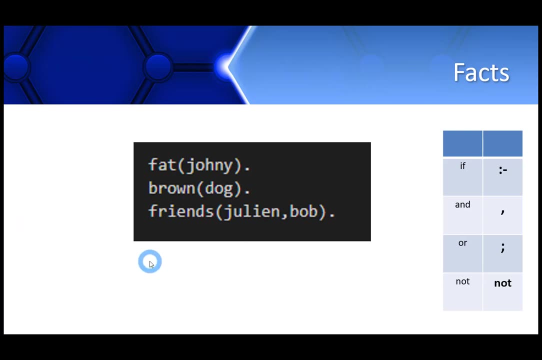 a single letter. it will be a capital letter. I have included this table on every slide so that if you see it again, again, you maybe you will memorize it quickly. now let's learn about some facts and rules. so previously we just learned about the knowledge base, and we learned that a knowledge base comprises of facts. 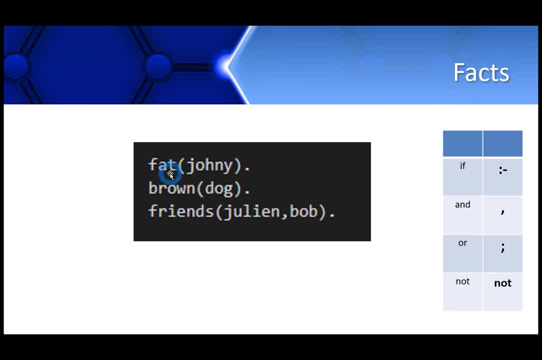 and rules. so let's take the example of facts first. so this is a fact and this is how I will write. I will actually write a fact in prologue. this is the syntax: how I will write a fact in prologue. so I'm gonna write the relation or the. 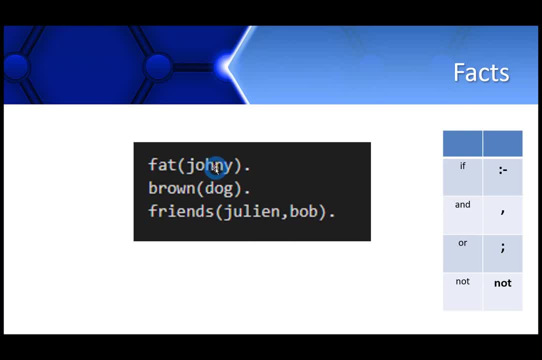 quality here and I will write the name in brackets here. so this particular line means Johnny is fat and dog is brown. Julian is French and I'm going to write Johnny as French and I'm going to write Johnny as French with Bob. this is how you read it and you always put a full stop at the 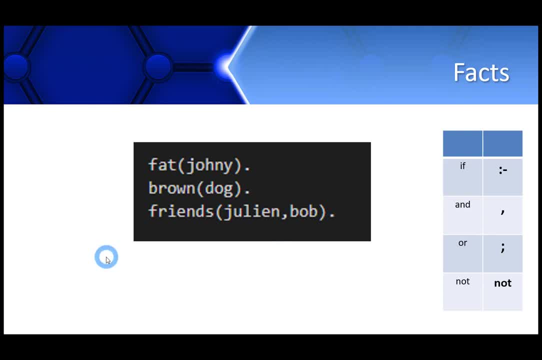 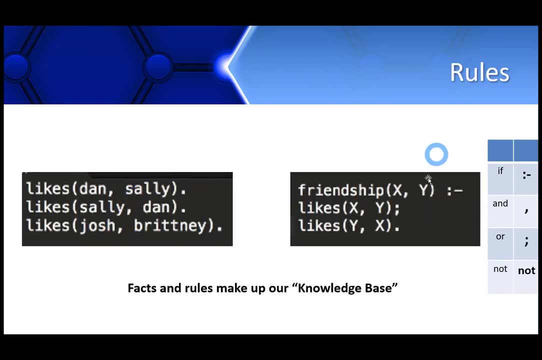 end of every statement in prologue. now let's see an example for rules. so okay, here these are my facts and this is my rule. so this is not a rule, this is a. these three are facts and this is a rule. now let's look at our facts. so the fact. 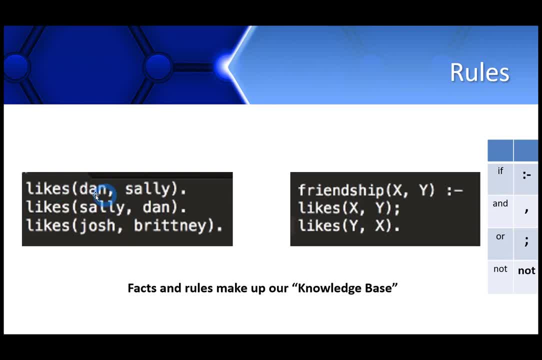 states that this person likes this person. so what I mean by that is: Dan likes Sally, Sally likes Dan, Josh likes Britney. So these are our three rules. Now let's see- sorry, these are our three facts. Now let's see the rule. So our rule states that there exists. 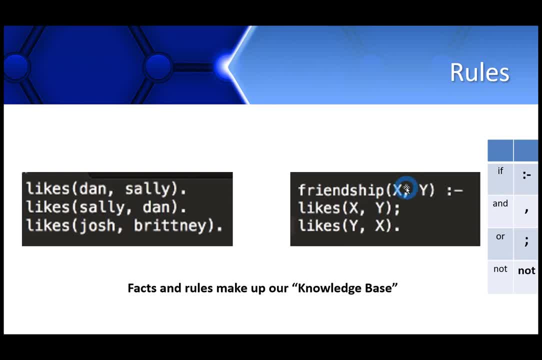 a friendship between X and Y, two people, X and Y. if so, this symbol is for. if you can see, here There exists a friendship between X and Y, if X likes Y. So what is this symbol for? You can see. 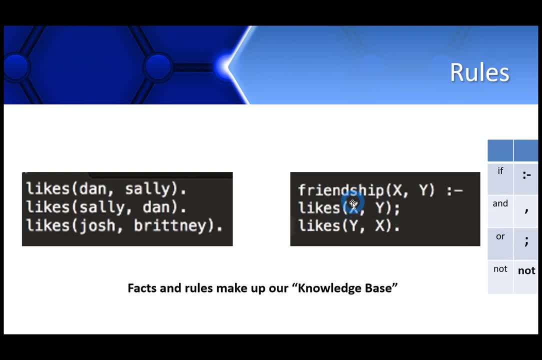 the symbol is for or So. there exists a friendship if X likes Y or Y likes X. So if either one of these statements is true, the friendship will hold right, If either one of these statements is true. So if I make a query about Sally and Dan, 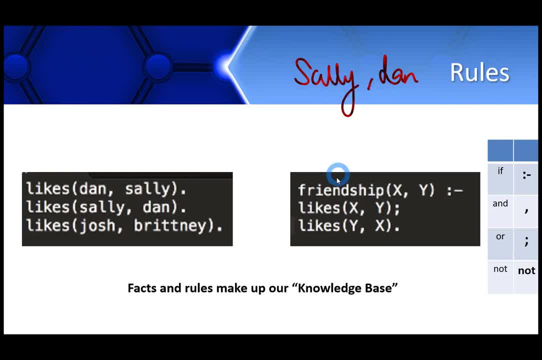 that, whether they like each other or not, I'm going to make a query about Sally and Dan, whether they like each other or not. I'm going to make a query about Sally and Dan. it will be true Why. Because the first statement X is Sally and Y is Dan. So the first statement 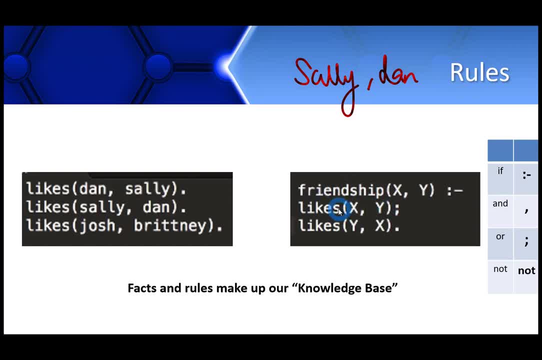 holds true in this case, right? So either if either one of these is true, the answer will be true. But let's say I change my rule and let's say I change it to. let's say I remove this or from here and I write, and instead of or. So now I have made a rule that the friendship between X and Y 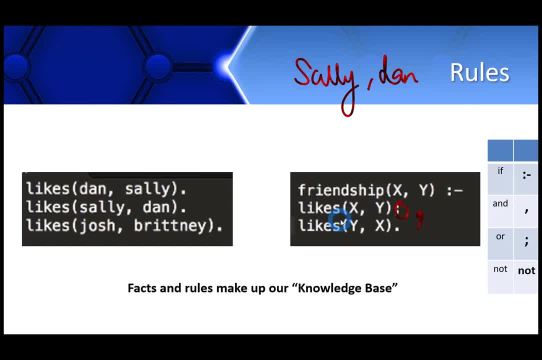 will hold if, and only if, X likes Y and Y likes S. So if both of X and Y likes each other, then the friendship will hold. If I change the rule to this, let's see Now if I make a query for this. 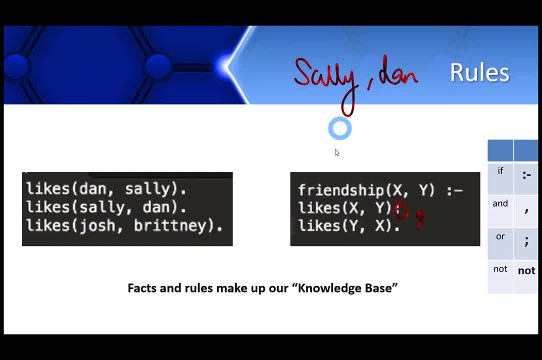 particular rule about Sally and Dan. it will be true. Why? Because a fact for both of them exists here. So Dan likes Sally and Sally likes Dan. So the fact, both of these statements are true, So their friendship will hold. But if I do the same thing for Josh and Brittany, the answer? 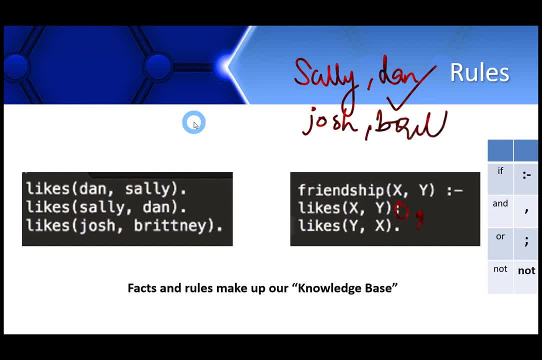 will not be true. Right? Why will it not be true? Because the statement for Josh likes Sally exists. First statement exists, but the second one doesn't exist. Since the second statement does not exist in our knowledge base, this means this rule will not hold this particular statement. true. 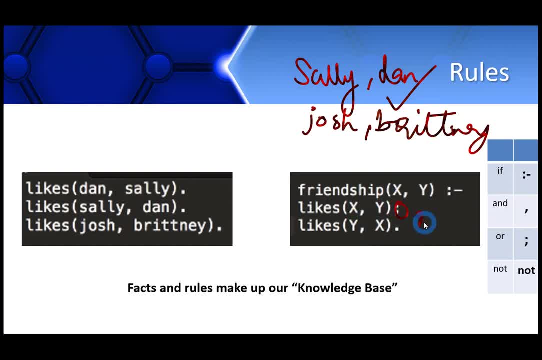 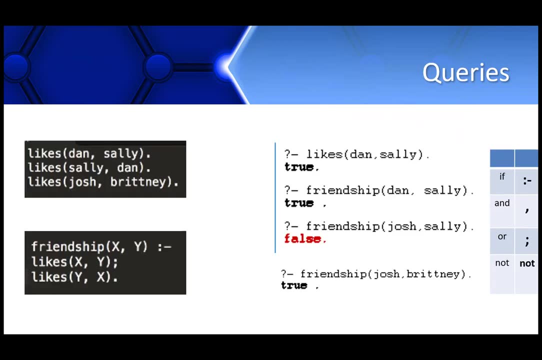 why? because in this particular rule, we were using and, and, and means. both of these statements must be true in order for this friendship to hold. right now, let's see some examples for queries. so this is the same knowledge base and this is our rule, and we have made different queries. so 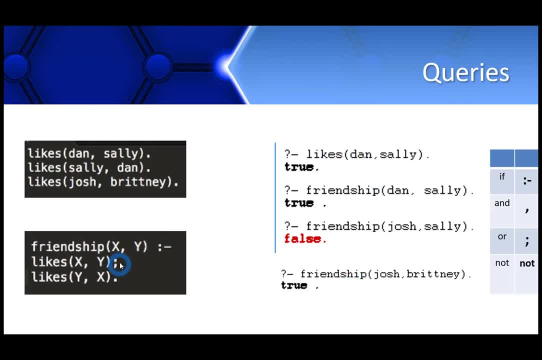 let's see the okay. remember this is or here. that means either one of is true. this rule will be true. so the first query is: does dan like sally? the answer is true because, yes, we have a fact for that here. the second query is for friendship does do we have a friendship between dan and?